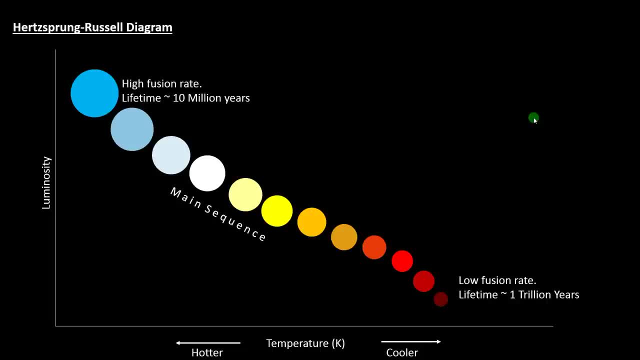 approximately a trillion years, so much longer than the age of the universe so far. And then we have stars somewhere in the middle, like our Sun, and our Sun should last around about 10 billion years, so it's about halfway through its lifetime at the moment. And then the other groups of stars we 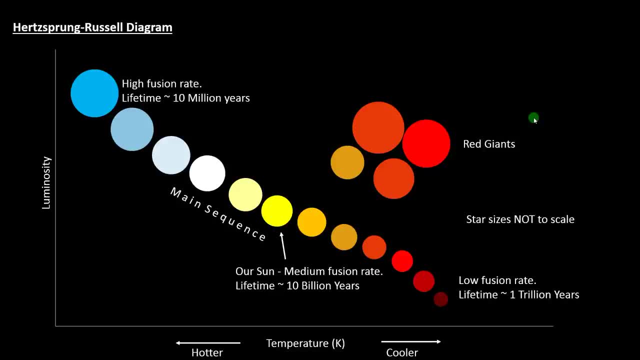 have are the red giants. so they're off to the little bit up and to the right on the diagram, so they are more luminous and slightly cooler than the sort of our Sun would be and larger. that's why they're called giants. and then we have 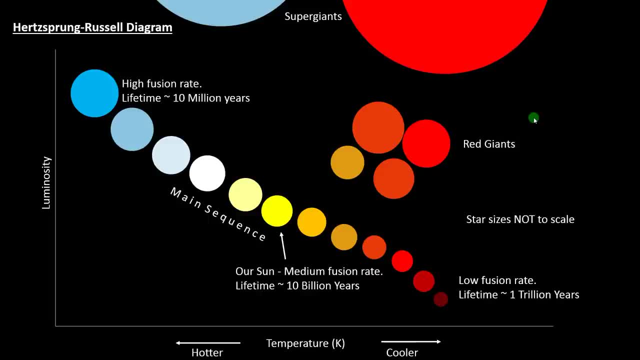 supergiants which are even larger and therefore even more luminous. above the red giants And the bottom left corner we have the white dwarfs. so you need to be able to label those sections of the Hertzsprung-Russell diagram, the main. 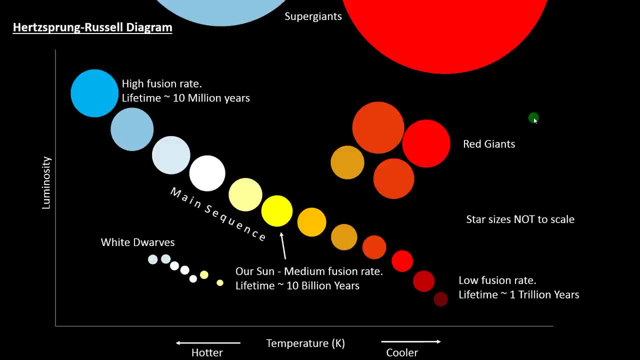 sequence: the red giants, the supergiants and the white dwarfs, And we also need to be able to talk about how two different types of stars evolve. you need to be able to do that as a sequence of descriptive writing, but you also it's useful to look at where they move on the Hertzsprung-Russell. 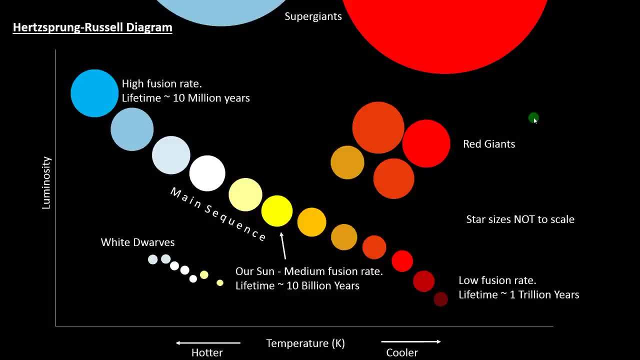 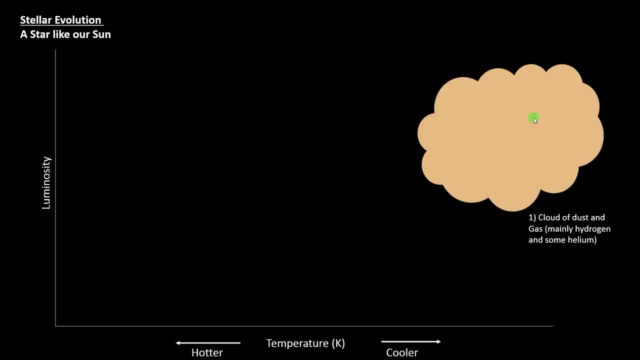 diagram because it will help to remember what's going on in the sequence. So the first one we're going to look at is a star like our Sun. We have to remember that stars form from collapsing clouds of gas, mainly hydrogen and some helium, and what happens is as the cloud 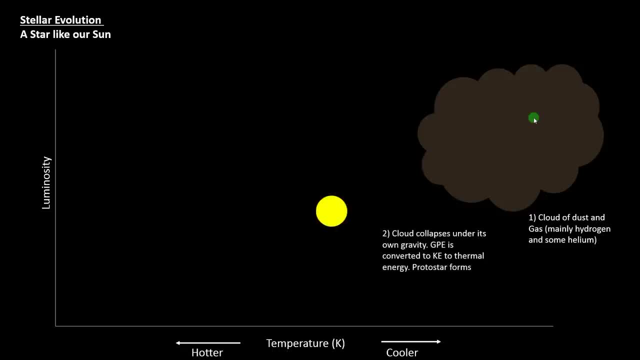 collapses. it collapses because its own gravity is pulling it together, so it's itself gravity pulling it together, and that means at the start it's got a lot of gravitational potential energy that is converted into kinetic energy as the collapse happens, and then all the collisions between the various atoms in 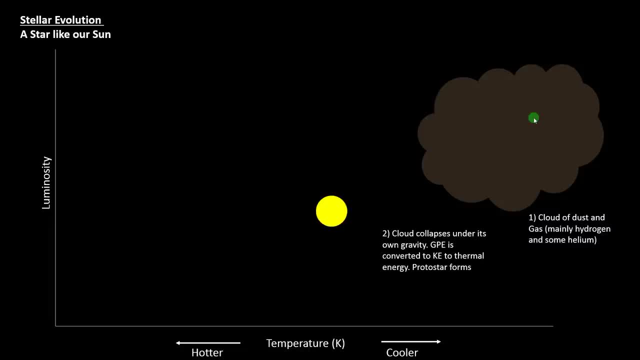 the cloud create, basically turn that kinetic energy into thermal energy and we get what's called a protostar, as fusion starts to happen in the core. Now you'll notice what happened was the cloud. initially was quite large and therefore had a reasonably high luminosity, even though it was quite cool As it. 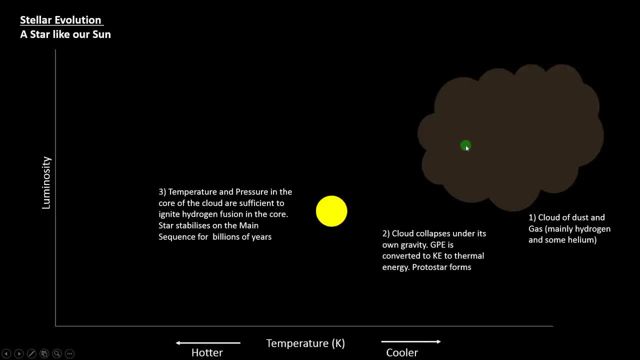 collapsed, the temperature increased but the luminosity dropped, and that's only because we've got less sort of surface area emitting light. As the cloud collapses, its surface area shrinks. even though it's hotter, its luminosity drops slightly. Okay, so once we get to the main sequence, then we've got: 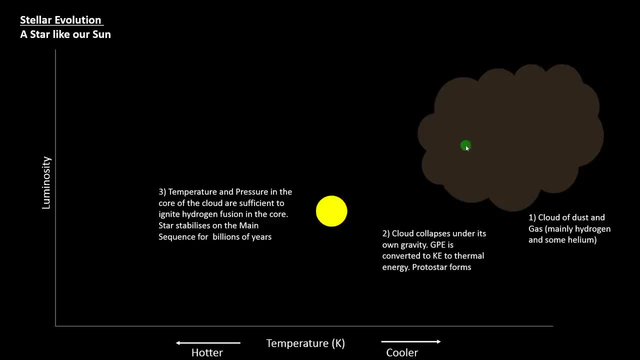 hydrogen fusion into helium going on in the core and the star stabilizes in this state on the main sequence for billions of years, like we've already seen. Okay, and what's happening here basically is that gravity is still trying to pull the star together, to together and compress it and the radiation pressure produced. 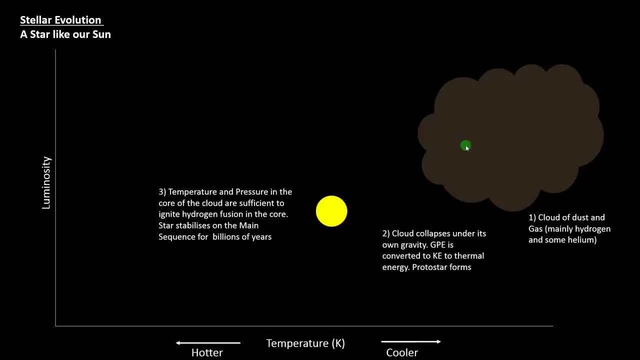 by the fusion process is pushing back out against that and the star stays stable whilst the hydrogen fusion is going on. But eventually the helium starts to build up in the core and the conditions for hydrogen fusion don't exist anymore where the hydrogen is, which is now a little bit further away. 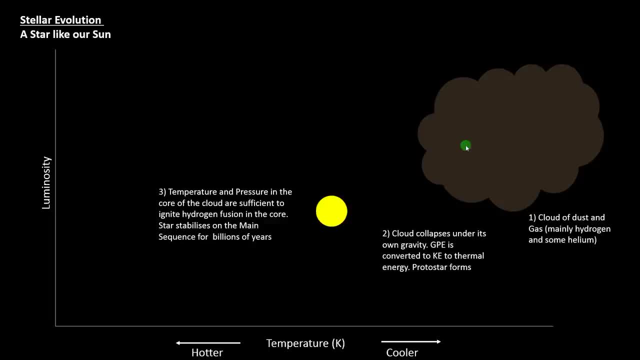 from the core because the helium is there, And when that happens, there's nothing to stop the collapse continuing of the star, and the core collapses first, and what we get is a core collapse and that core collapse again releases a lot of gravitational potential energy into thermal energy. 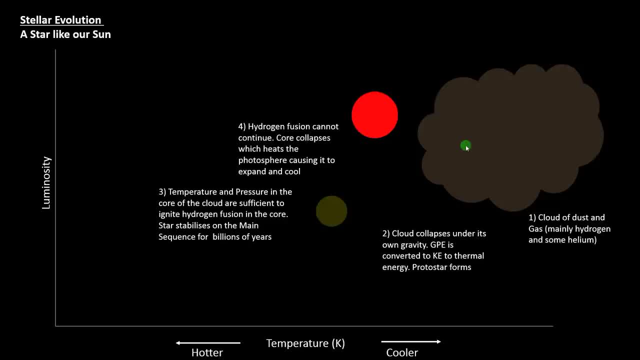 which heats the outer layers of the star, causing them to expand. The photosphere is the outer layer of the star where the light is emitted from. Those outer layers expand and they will eventually cool and that's why we get the red giant. Okay again. the luminosity is increased from the main sequence. 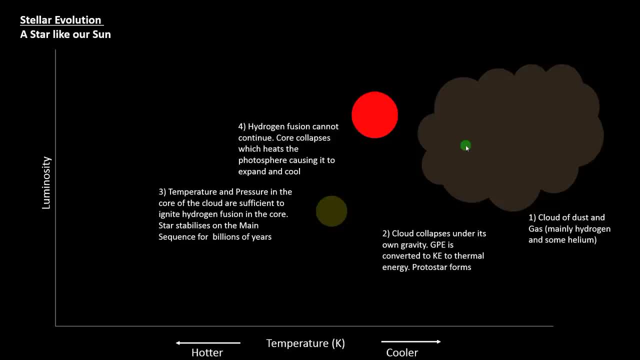 the temperature has decreased slightly because the photosphere cools when it expands. So that's the red giant. and what's actually going on there is that now, instead of fusing hydrogen into helium, we are now fusing helium in the core to elements like carbon, nitrogen and oxygen. Okay, that's something called. 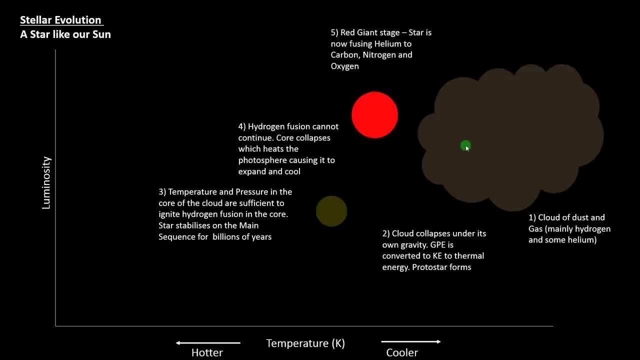 the CNO cycle that happens in these red giants. Now, a star like our Sun doesn't have enough mass to fuse beyond those elements. Okay, basically, to get further along the periodic table in fusion, you need a star of larger mass because you need higher and higher temperature and pressure to get the next. 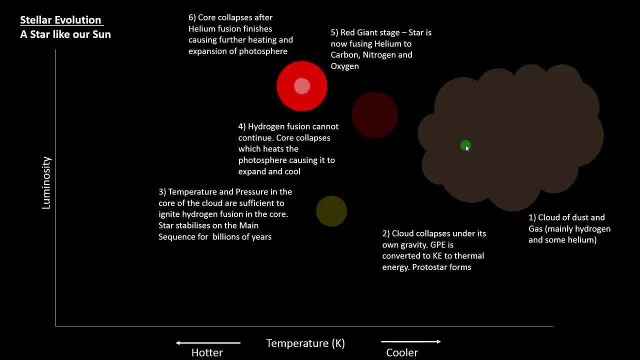 fusion reaction to happen along the sequence. So what happens at the end of that fusion is that the core collapses even further and it heats the outer layer so much that they swell up even more and they are basically blown off the star in this shockwave and form what's called a planetary nebula. So just show you that. 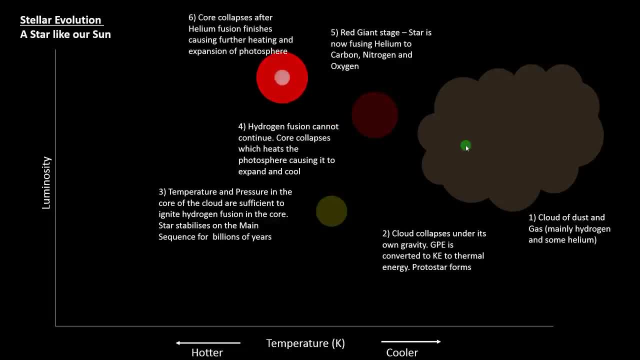 one more time. there's the red giant star. Okay, the core collapses, the outer layers expand even more and they're just blown off the star. okay, now, what's happening to the luminosity during that point is due to the heating of the. thanks to the core collapse, the luminosity 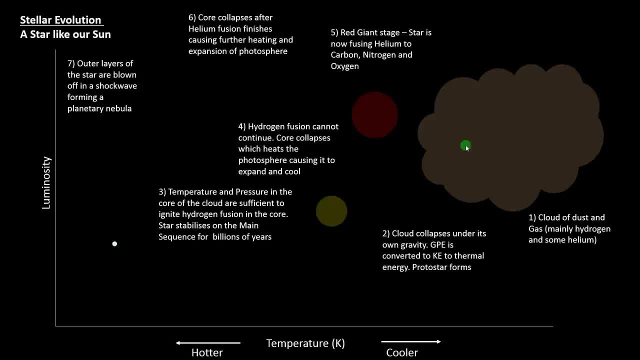 increases initially as the star is getting larger and slightly hotter, and then, when the outer layers are blown off, they're not really part of the star anymore and all that's left is this very compacted core which forms basically the white dwarf. now it's very, very hot, which is why we're over on the. 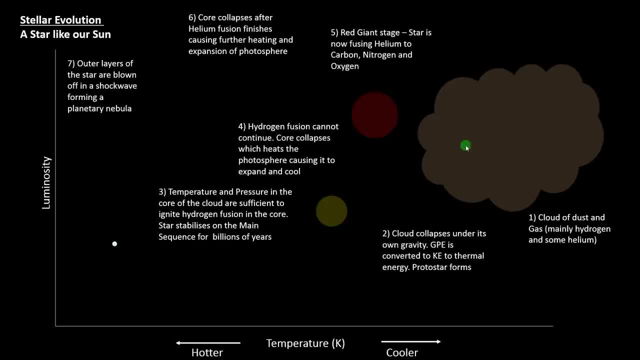 left hand side of the diagram, but its luminosity is quite low because it's so small. there's not a lot of area to give out the lights. now, during the white dwarf stage- this is the important thing- no more fusion occurs. it's fused as far as it can. it can't create the conditions for any more fusion. 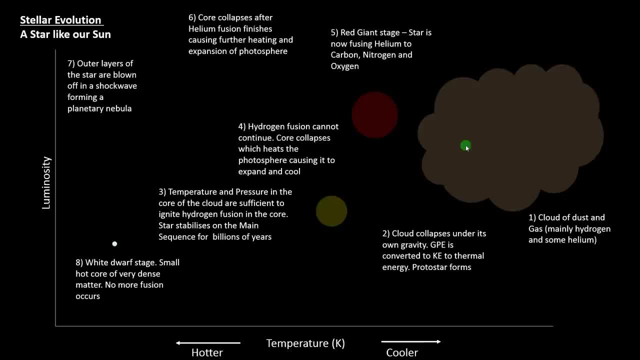 so it's not releasing energy that's locked up in nucleus of the nuclei of the atoms in that star anymore. so as a result of that, all it does now is lose the energy it's got and it gradually cools down. so that white dwarf will cool down. it will get less luminous because its temperature is dropping. 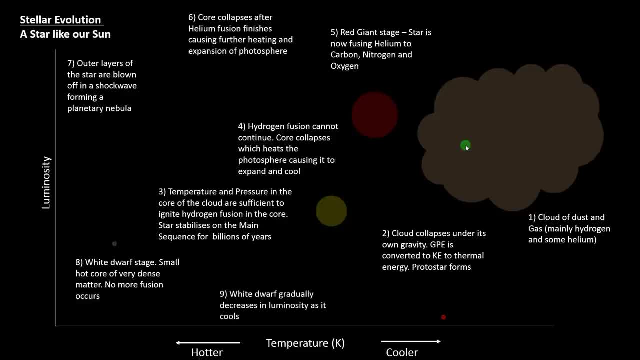 it will go to the right on the diagram because its temperature is dropping and it sort of cools and fades away and eventually it's very difficult to detect it at all because it's hardly giving out any visible light. so that's the sequence of events for a star that is similar to our sun. 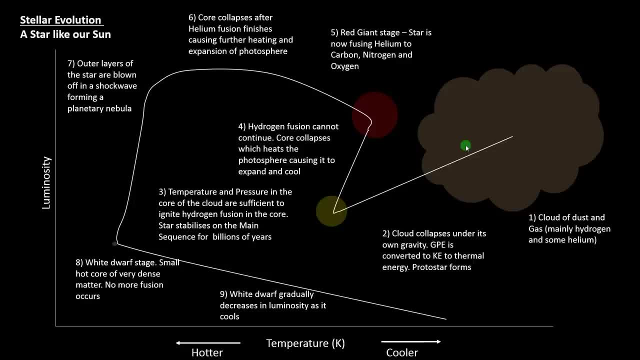 okay, you need to be able to reproduce part, whole or parts of that. a six marker might not ask you about the entire process, but it might ask you to explain what happens to a star like our sun forever from the main sequence, in which case you go from step three and you wouldn't worry about step one. 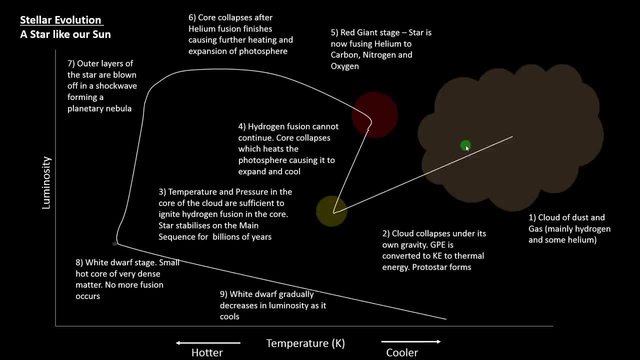 and two. it might ask you to describe the formation of the star and what happens to it, up to the red giant stage. so you need to be able to pick sections out in order to focus on the marks that you're going to need to get for the six markers. okay, so that's a star like our sun, the other one you need. 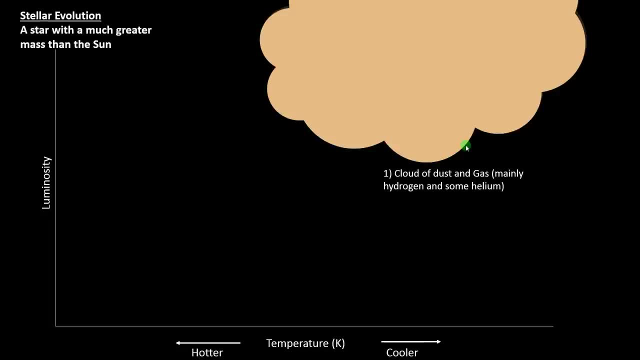 to know, is a star that is significantly heavier than our sun, so we'll look at that on the diagram as well. again, we start with a cloud of gas, mainly hydrogen gas, and then we start with a cloud of gas and helium again, and this cloud is obviously much larger because it's going to produce a larger star. 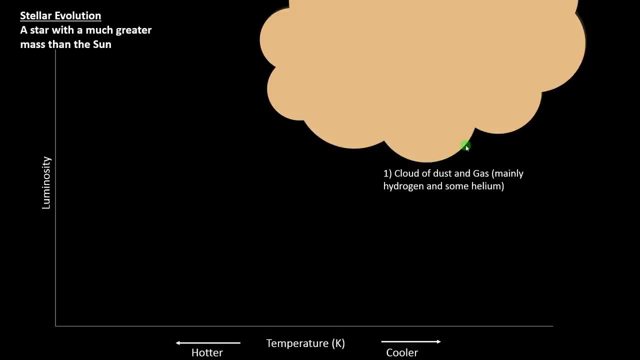 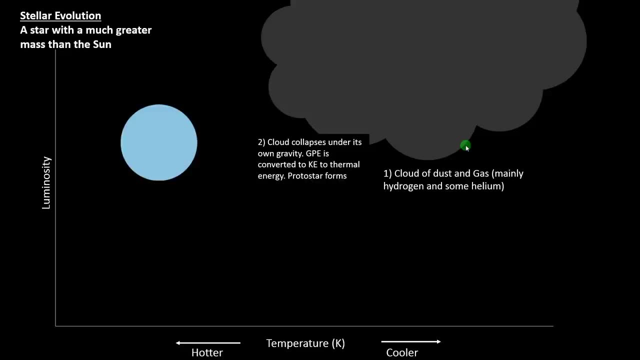 again, it's very luminous, even though it's relatively cool, just because it's so big. as it collapses, the luminosity drops, but the temperature increases again. due to this same process of gravitational potential energy being converted to kinetic and then to thermal, we get the protostar. 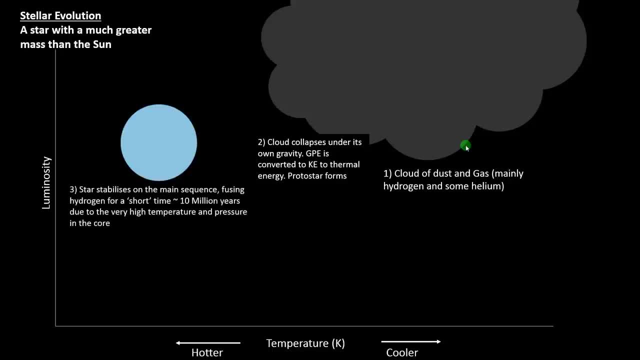 and the fusion starts to happen. and then it stabilizes on the main sequence again for a much shorter period of time. because the star is more massive, the fusion rate is much higher. okay, but again, once it can't fuse hydrogen anymore into helium, it does the same sort of process as the 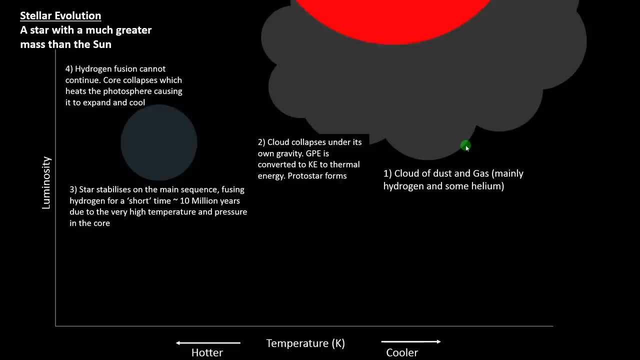 our sun would do, except, instead of swelling to a giant star, it swells into a super giant. okay, but the same basic idea is. up to this point, the star is now fusing helium into carbon nitrogen and oxygen. but what it can do- which our sun couldn't do, or a star similar to our sun- is that 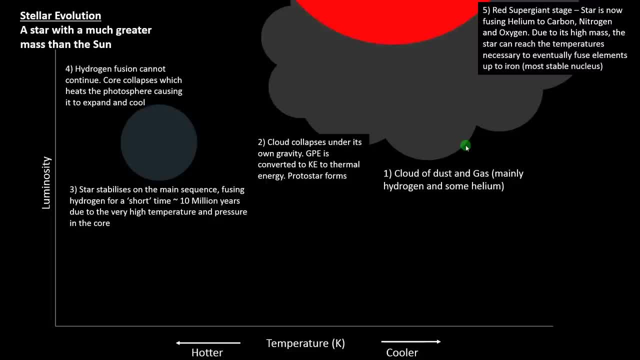 this star has enough mass to create the conditions, the higher temperature and pressure needed to fuse past carbon, nitrogen and oxygen, and in fact it can fuse all the way up to element number 26, which is iron. and iron, it happens, has the most stable nucleus of any element. so once it, 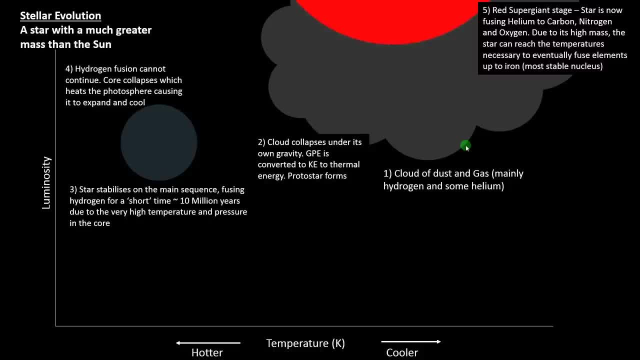 gets to that point, it's impossible for it to release energy by fusion anymore because it's at the most stable point. so, even though it can create these higher fusion reactions, we again end up with a situation where the star is not able to maintain fusion and because of that it will collapse, because 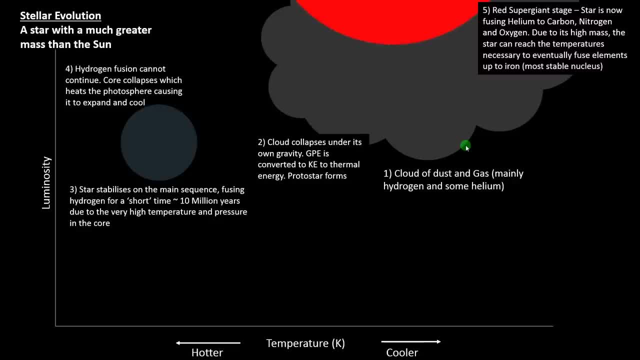 there's no radiation pressure anymore. the collapse here, because the star is much larger, is much more catastrophic. the star essentially completely collapses itself in a very, very short amount of time and we get a supernova. so that star is now vanished. the reason i've not shown the supernova: 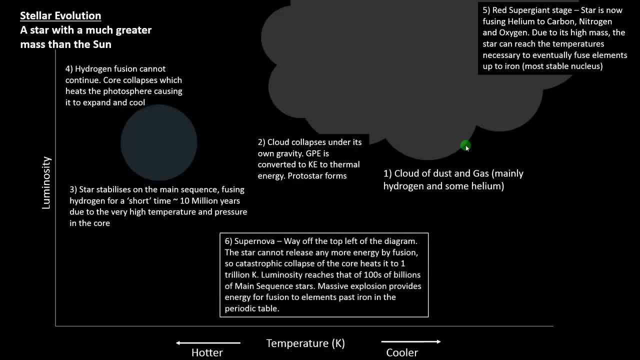 is because the supernova is so bright that it's way off the top left of the diagram. okay, it is incredibly hot- a trillion degrees kelvin- and it is incredibly bright. um, a supernova in a galaxy can typically outshine all the other stars in that. 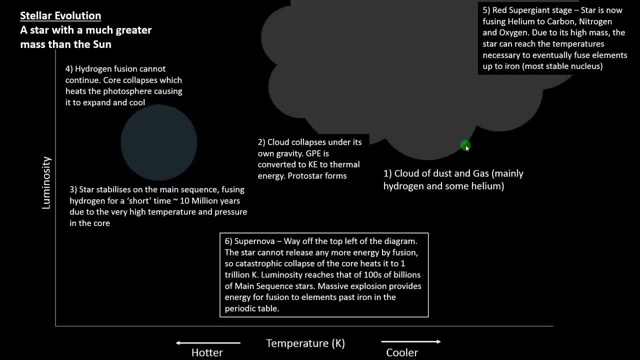 galaxy during its initial phases. so hundreds of billions of main sequence star brightness. okay, and what that does is, if you think about it, in the early universe we had hydrogen helium, but all the other elements have come from somewhere. we've got explanations so far for where everything up to iron. 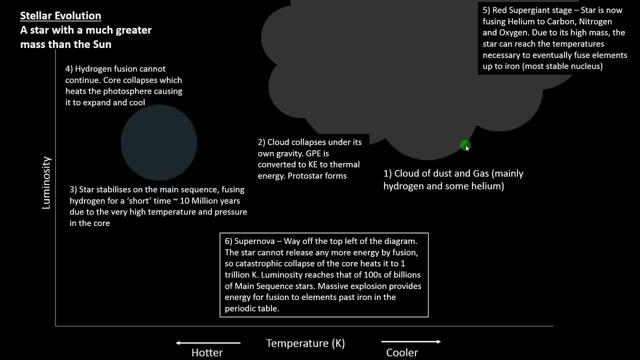 has come from but the. the gravitational energy released in that massive collapse of the core of this huge star is enough to actually put energy in to fuse elements past iron in the periodic table, elements past iron past, element number 26, were created in supernova explosions. okay. 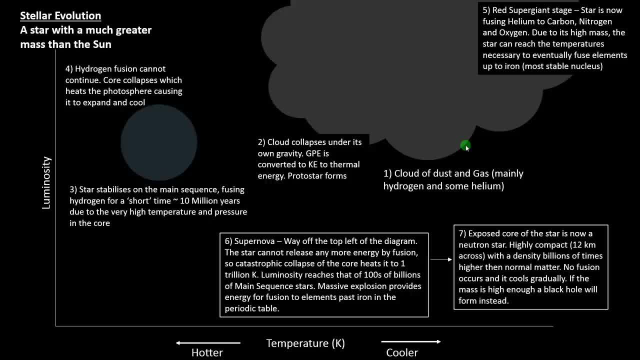 and then what happens then is that the the gravity is so strong here that we get what's called a neutron star and basically, if you think about a normal atom, it has protons, neutrons and electrons, and a normal atom has an equal number of protons and electrons. the gravity is so strong in this. 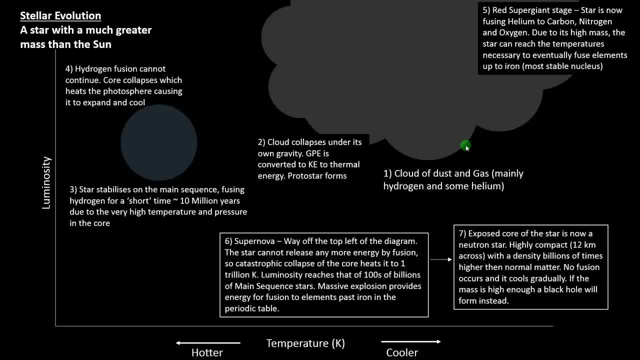 situation that it forces the electrons into the protons and turns them into neutrons, okay. so it's kind of like a reverse beta decay, okay. what that basically turns the star into is a giant atomic nucleus, 12 kilometers across, roughly neutron stars. but it's all nucleus, there's none. 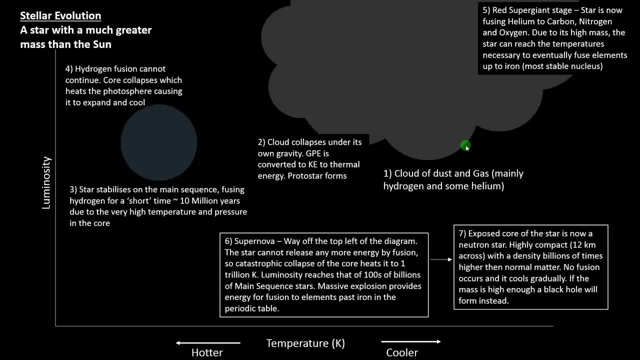 of the gaps that you have in a normal atom between the nuclei. that means it's incredibly dense- billions of times the density of normal matter- but again we're in the same situation. it can't release any more energy by fusion. it's incredibly hot to start with because it's so small actually. 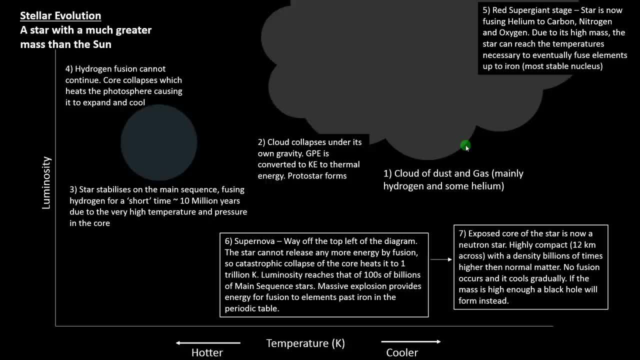 then the, the. we can't plot the neutron star on the hertz spring russell diagram because despite its massive initial temperature, it's so small that its luminosity is very low. so it would actually be off the bottom left of the diagram and it does a similar thing to the white dwarfs. it will cool. 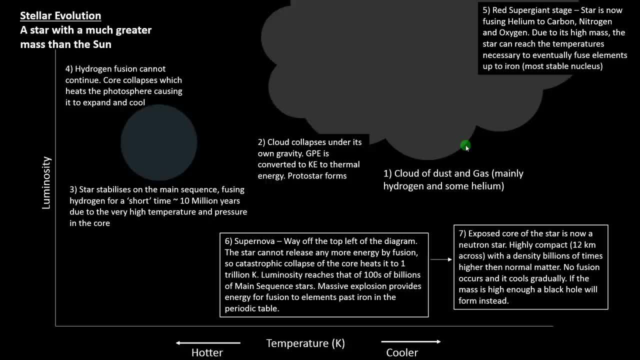 gradually okay, and eventually, once it's completely cooled, it won't be visible anymore. the other thing you need to know is that is the alternative final stage. if you have a star that even higher initial mass than one, that will form a neutron star and you're in the same situation. but if you have an 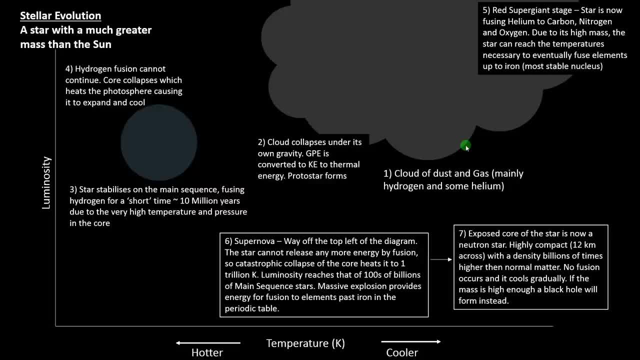 star, then gravity is so strong that it even compresses all the neutrons together and you get a black hole. and nobody really understands what exactly a black hole is in terms of what's inside it. but the reason it's the black hole is that the gravity then is so strong at what we 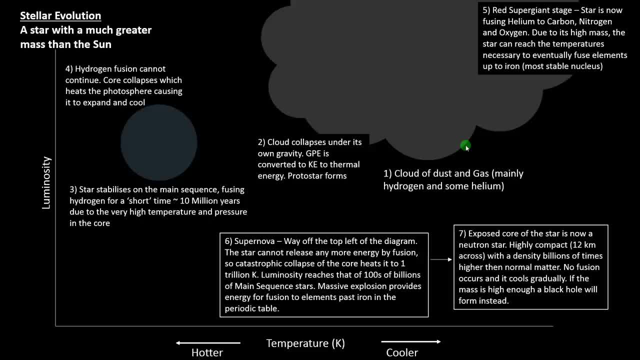 call the event horizon on the surface of the black hole that not even light can escape it, so that's why it's black. So there are the two types of stellar evolution that you need to know. certainly worth remembering how the first one fits on the Hertzsprung-Russell diagram, as you.